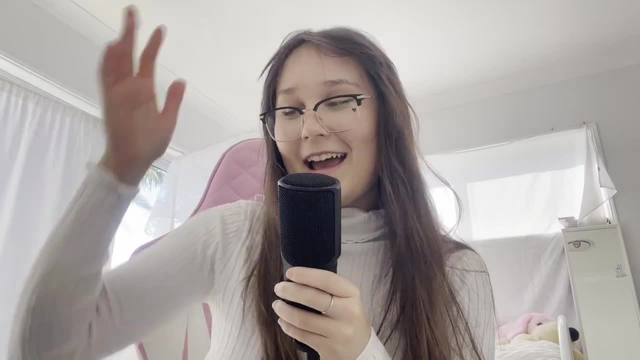 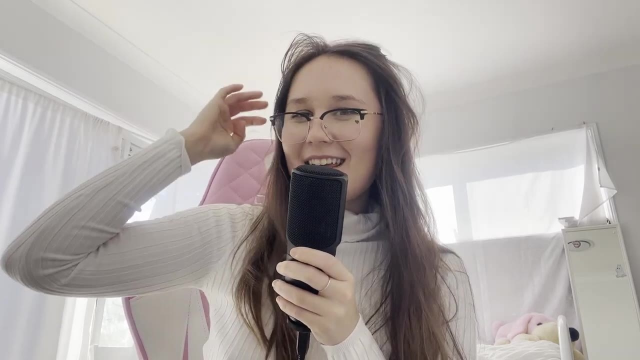 to the ideas. Okay, I'm just gonna be reading them out and just seeing how we go. This is so exciting and just like so fun- being able to talk about all these interesting ideas- and they're kind of just like prompts sort of things, um for you to maybe take or get inspired from. So let's get on to it. 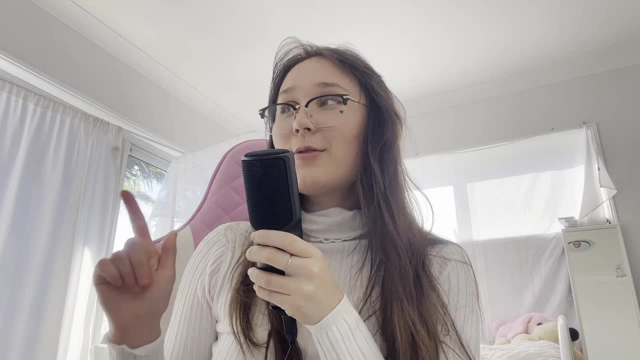 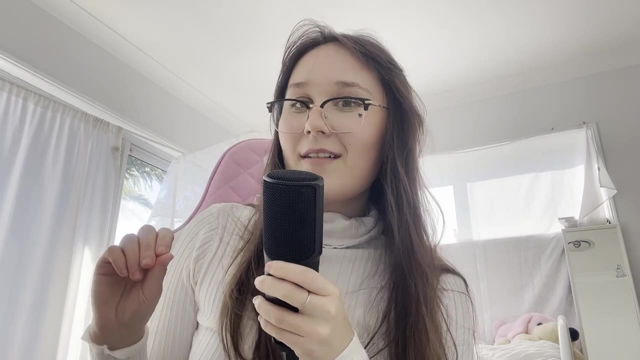 because the first book idea is a wholesome dragon trainer who lives in a a wood in the woods with a dragon. So I'm going to be reading this book and I'm going to be reading this book and with his wizard uncle. So I don't know, this is just like a fun, like I wasn't really sure about. 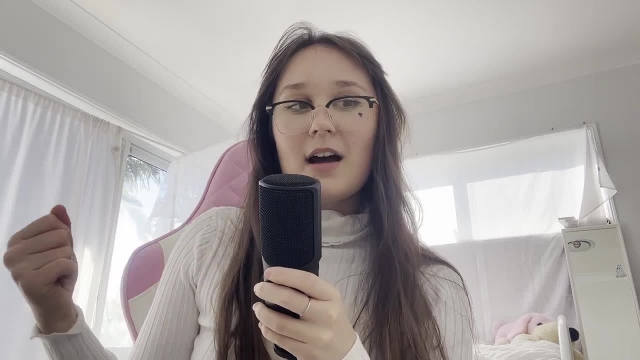 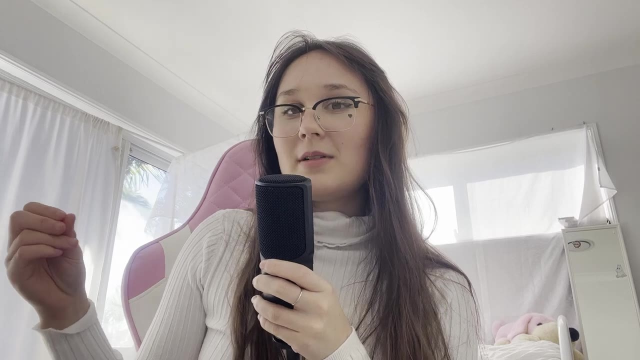 this book idea like what can be like the, the main incident, um, but maybe like, the woods ends up getting caught on fire and then the dragons are in danger or something. or maybe someone kidnaps his um uncle, The dragon trainer's uncle, or something like that, and then he needs to, like, use his 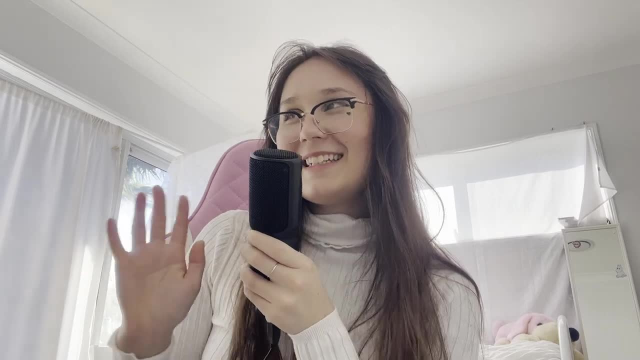 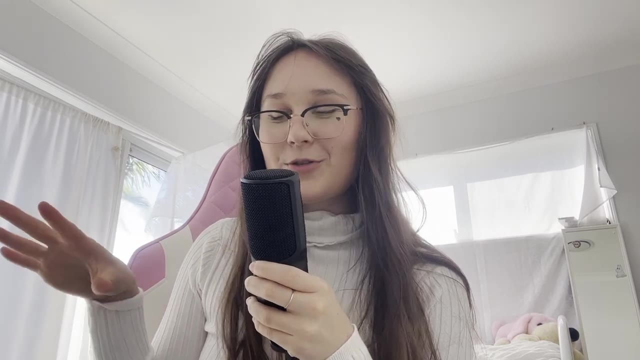 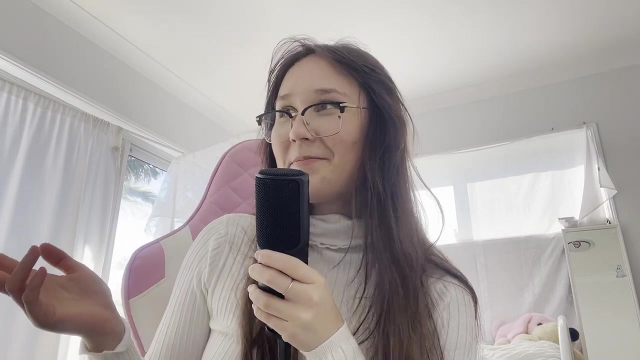 dragons to help find him or something like that. um, but yeah, I thought this was a really cool idea, really wholesome, very like uh vibey in a way, where it's like you can see the mushrooms and the dragons, especially with Fourth Wing, which is a very popular novel at the moment. um, but yeah, that's one of them. The second: 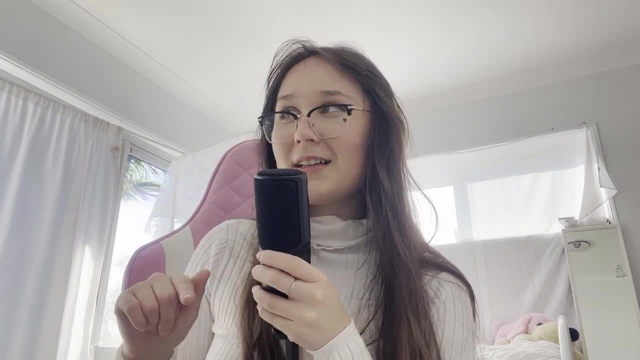 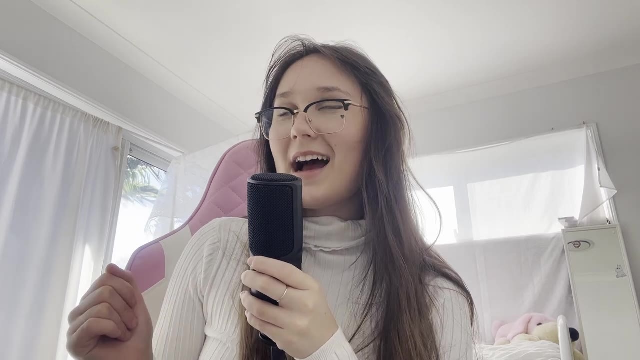 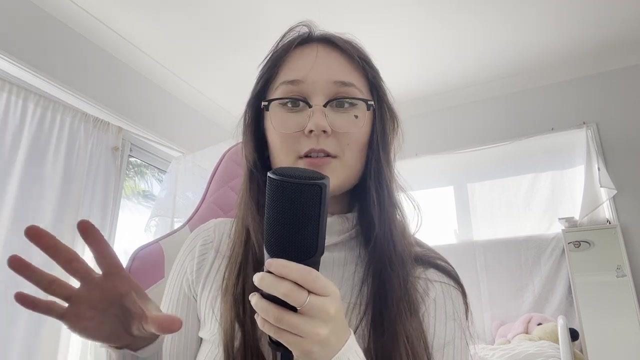 book idea is a sculptor who has the ability to sculpt ghosts, capturing their spirits. This seems really interesting and I don't know, I was kind of like really intrigued with this idea because I have written, actually a short story which includes a sculptor, and I think sculptors 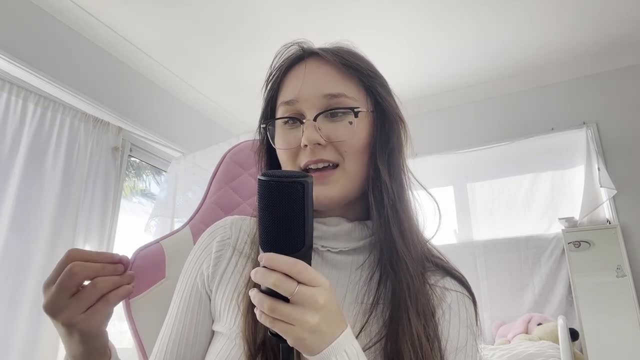 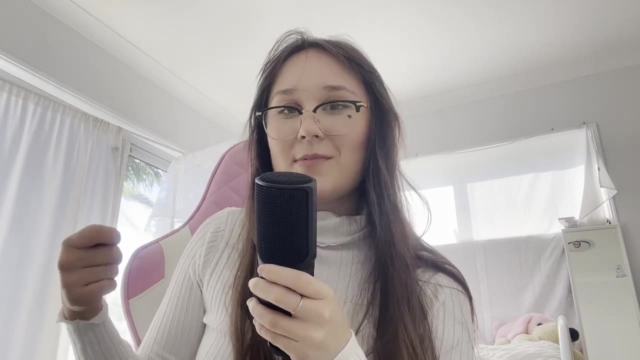 as artists are so interesting and the fact that, like I don't know, maybe they can see ghosts, like this sculptor can see a ghost and sculpt, you know the ghost and like their story, but also capture them and like, harness them into the stone so that they kind of materialize into real life and maybe 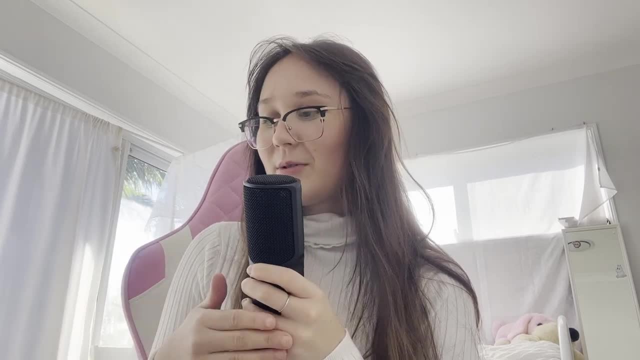 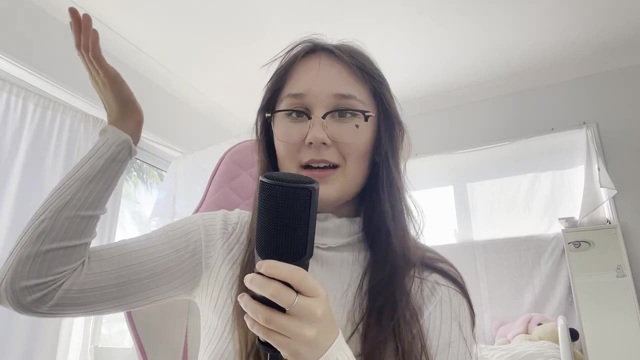 that has a lot of you know sorts of problems, or maybe she falls in love with one of them, I don't know. maybe they can talk to her cool fun things. the sculptor can be a guy as well, but um, I just kind of always imagine. 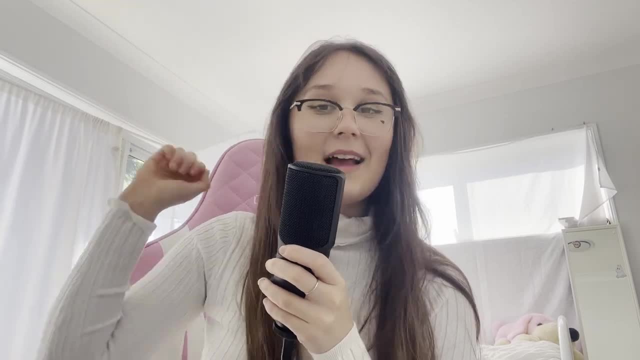 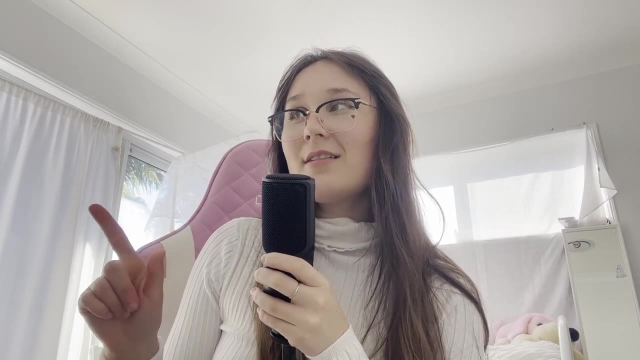 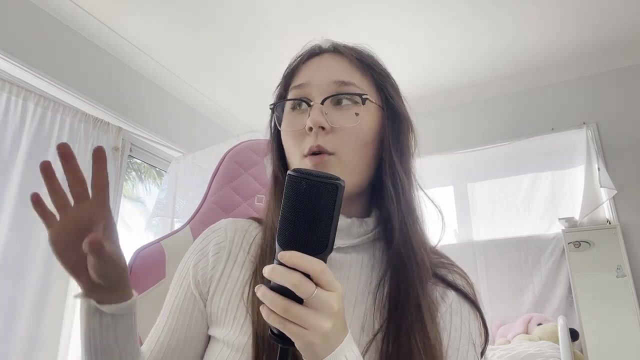 A really cool woman sculptor. anyways, that's that idea. um, let's continue. the third book idea is a long lost and missing princess who was trapped in a mirror. I got this and, by the way, all these ideas are basically inspired by a board I have. that's just like random book ideas and paintings. 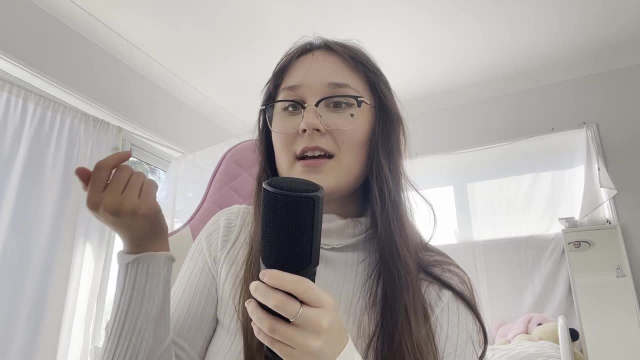 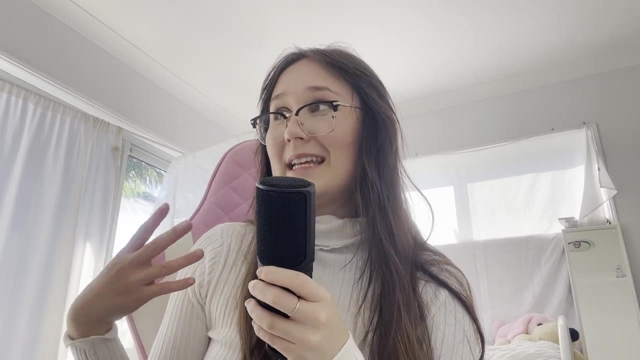 and like photos literally just inspire these, like, just like that. so I had a photo of a, a princess, looking into the mirror. you can't see her face, but like, maybe she's trapped in the mirrors and people think that she's lost, when she's really just lost in her own castle. how cool would that. 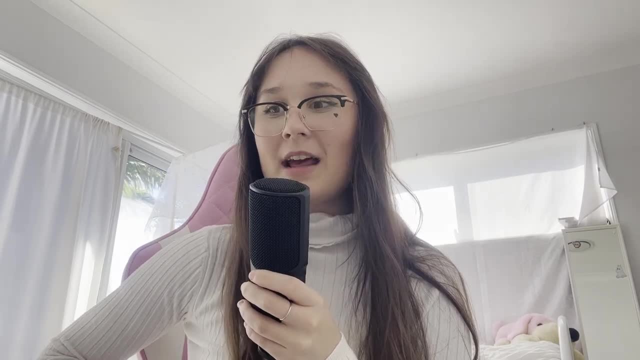 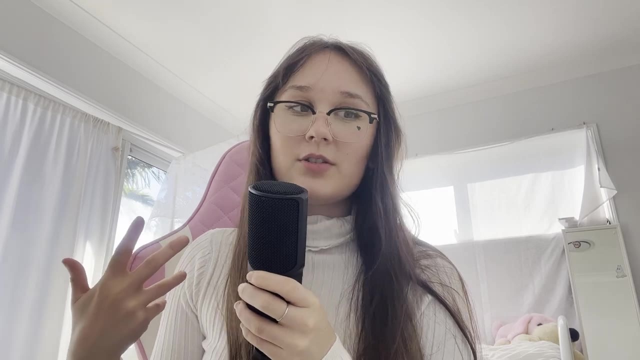 be and somehow she needs to get out and maybe, like someone ends up helping her or she actually gets transported to a new place, maybe because she gets forgotten, you know, she starts to disappear or something. that's something you know. it has like that sort of kingdom-esque vibe, but also 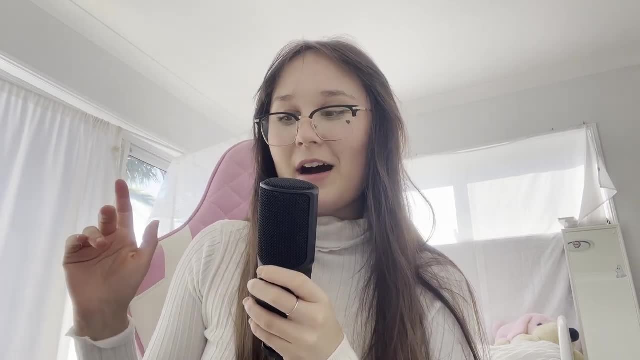 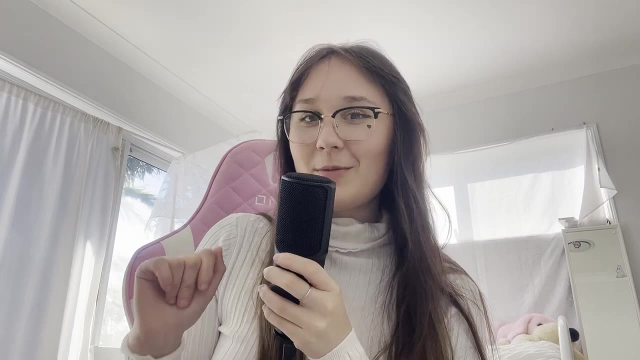 like a little bit of like a mystery, sort of um Thriller, like oh, I don't know, but that's that. next up we have a boy who falls in love with a shadow. I was gonna say something like to do with his own shadow, like maybe he befriends his own. 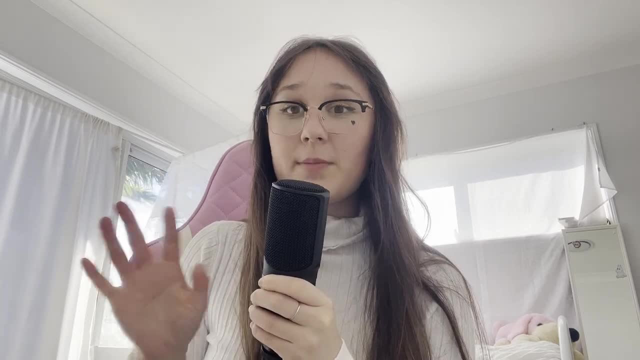 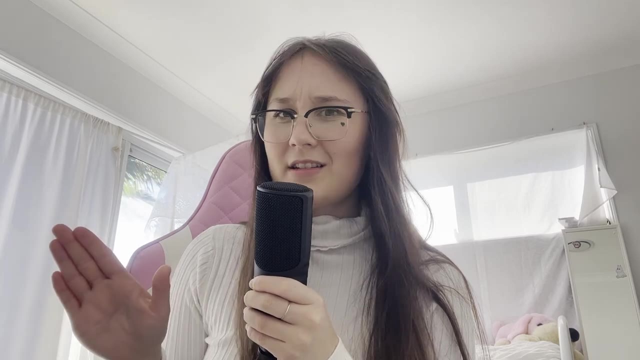 shadow, like because I'm really inspired by um Peter Pan and his relationship with his shadow and his shadow like being like a mother to him, sort of thing. um, it's so interesting to like research. I love Peter Pan, so like maybe something like that. but maybe he falls in love with like 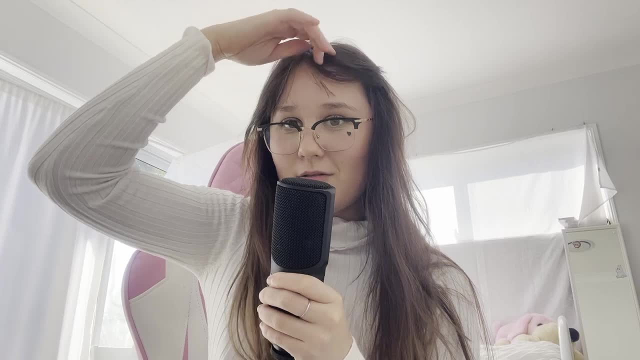 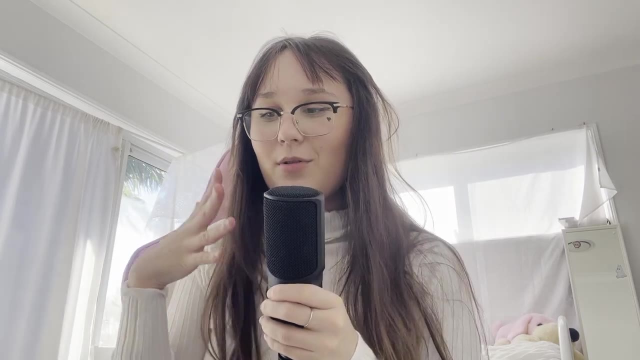 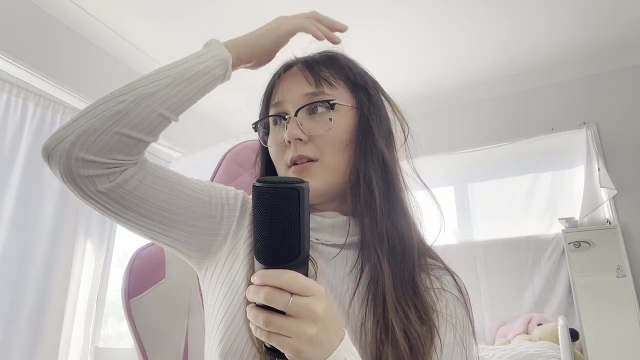 someone else's shadow, but not like The person who casts the shadow, I don't know. just like interesting thought like that, like I don't know. it seems like again like that sort of vibe I love, like my ghost story, sort of um novel, like that sort of vibe is exactly what I love. so a lot of these ideas probably. 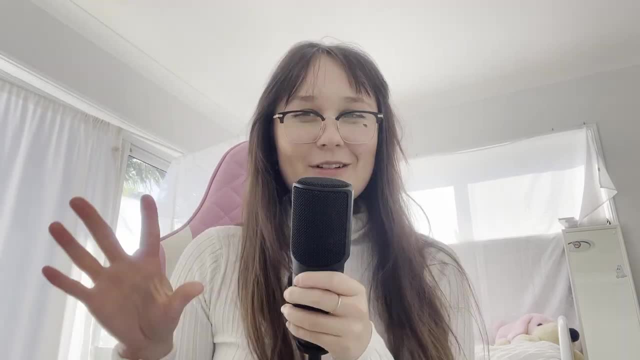 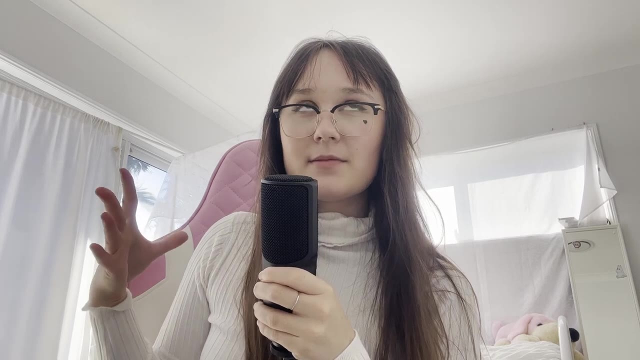 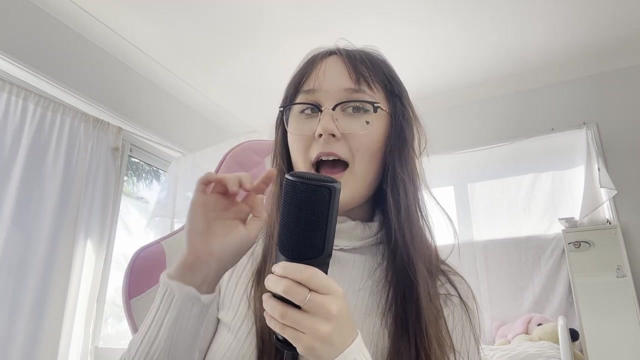 go with that, but I tried to include, like the first one, more like foresty fantasy ones, so let's continue. oh, this is more of a um, like real, uh, dystopian sort of one. um, if you guys- I don't know if you guys also, this is a little bit of a tangent if you haven't watched- 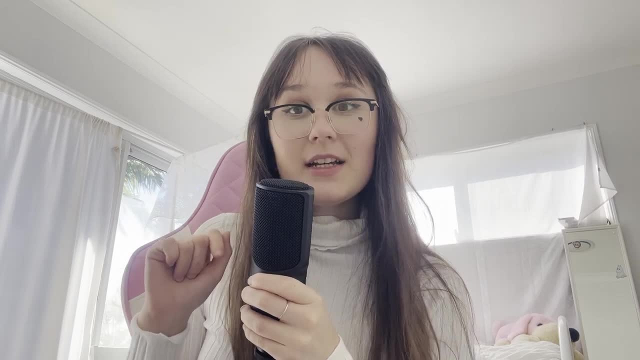 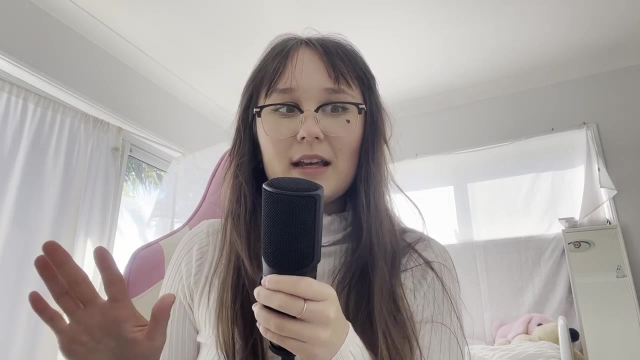 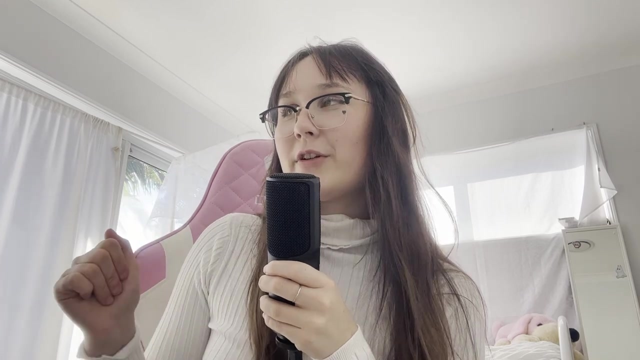 um love, death and robots on um Netflix. it's such a good show. there's just like really random, like 20, even like 5 to 10 minute like episodes which are so interesting and this like gives the vibe, and I did get like a little bit inspired by like a few of their short films. um, it's so good watch. 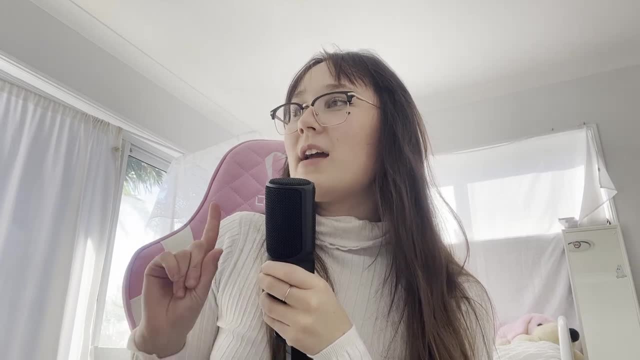 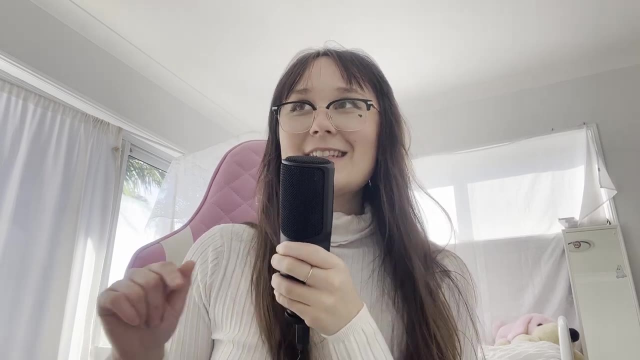 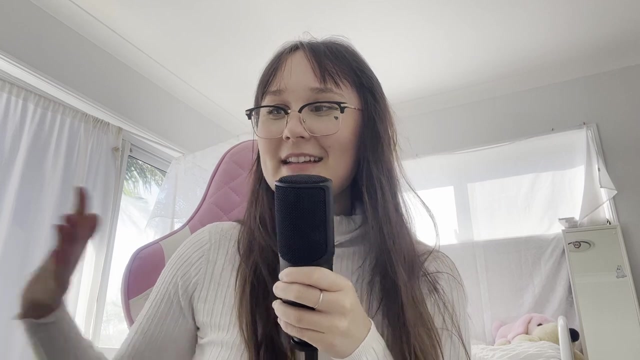 on netty Netflix. but this is where a pilot trainer crash lands when he finds a traitor sleeping in his cargo or like some, like a villain sort of you know, or like a random person who actually is like on the other side of the war or something. but they end up like 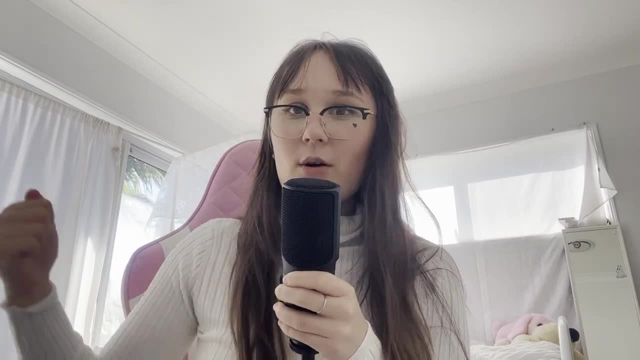 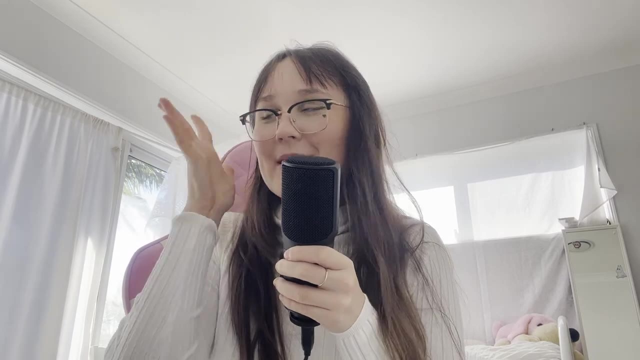 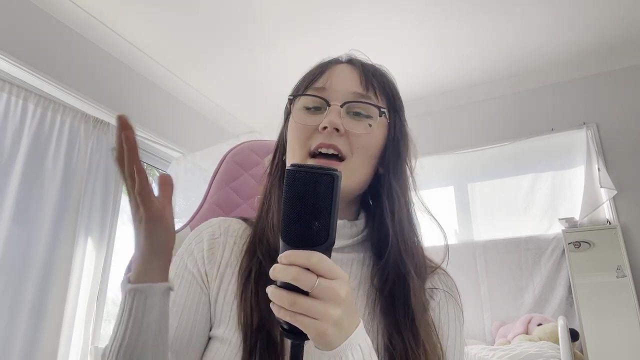 having to- you know, band together to get off the planet that they crash on, maybe, or like a desolate place, something like that. I don't know, you cannot hear what I just said. um, I'm just so excited, um, but that'll be so fun. I've always wanted to try like a sci-fi, more dystopian, um, like a. 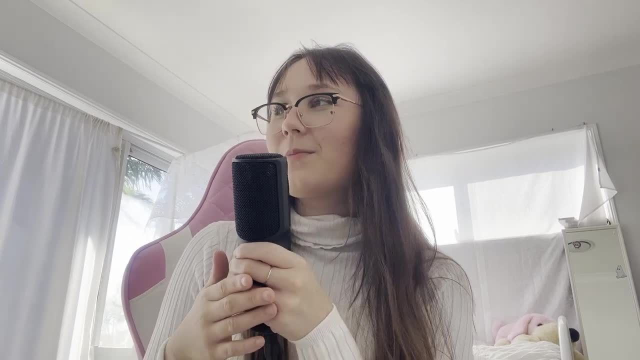 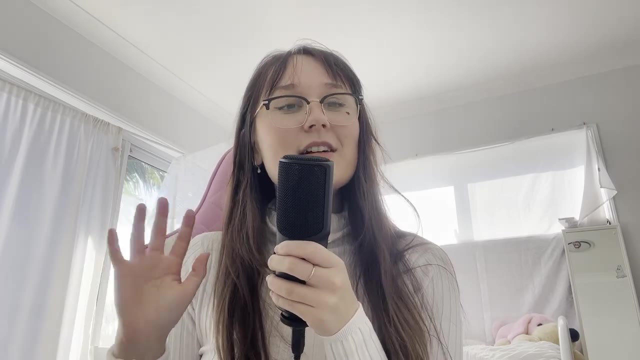 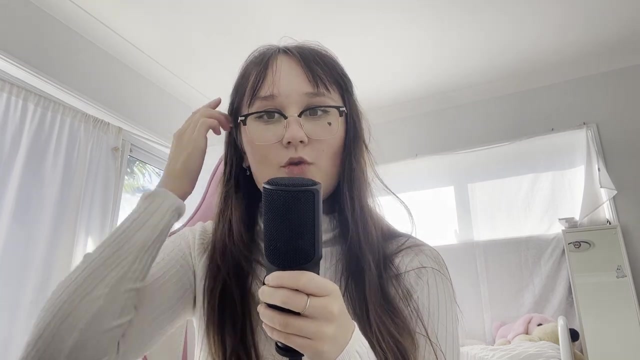 dystopian sort of book because it just seems so intriguing. okay, let's continue. a boy who talks to crows and is able to communicate with crows: I have such an interesting short story, kind of similar to this, to do with crows and birds, because I'm obsessed with birds. I used to only like draw. 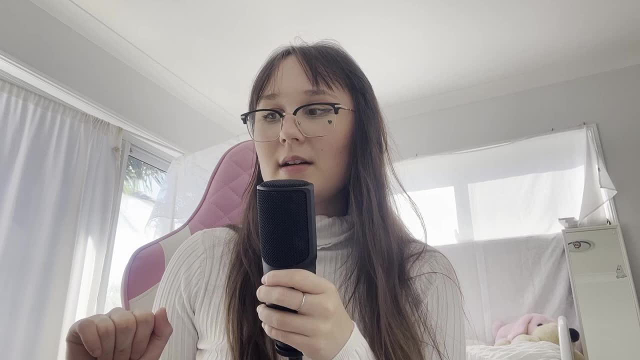 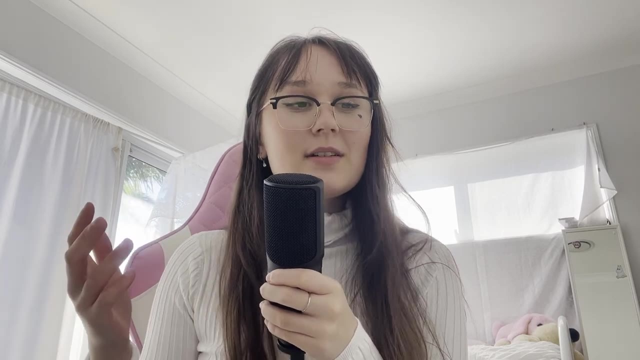 birds when I was little- I just like draw so many birds- but also in a lot of my books- I think I've talked about this before- where, um, the main character- at least a character or a sort of motif in the book- is some something has to do with the character or a sort of motif in the book. 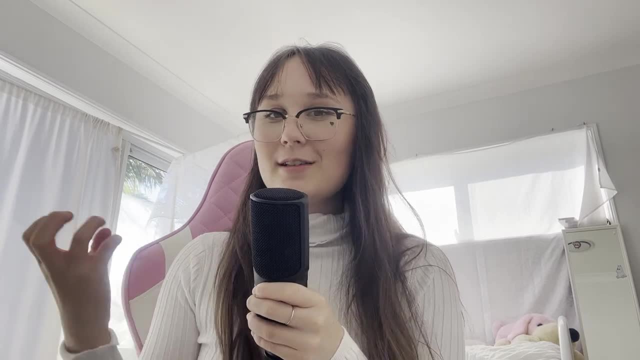 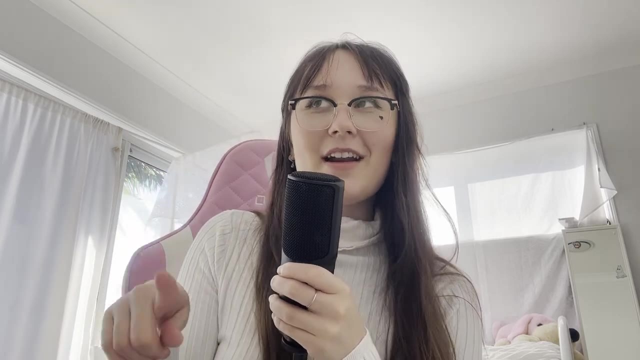 and that's in like all of my books. basically, somehow, I always allude to a bird, so that's why I just love birds in general. um, if you didn't know, my favorite bird slash kind of favorite animal is a pelican. I love pelicans. so, yeah, that's that one. okay, next up, a trained assassin. 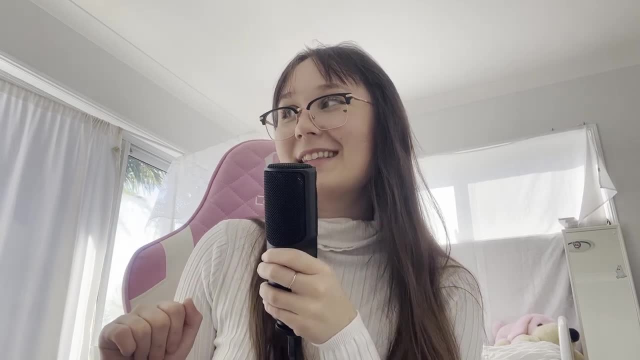 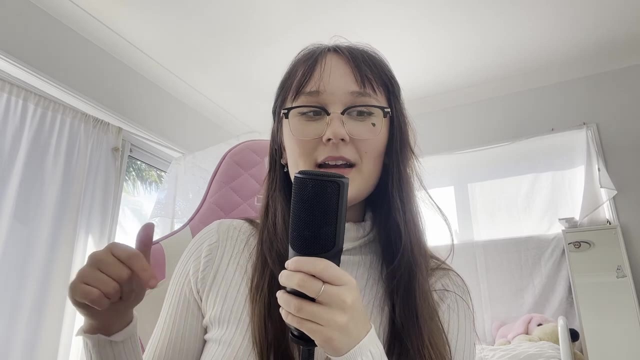 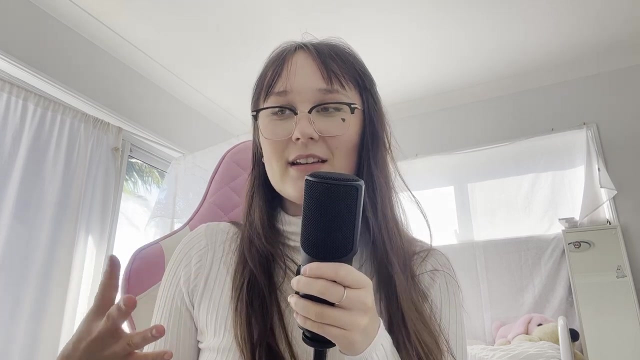 is tasked with protecting a petty prince who turns out being an assassin himself. this is actually a book idea that I had a little bit while back in a little um photo just kind of sparked that. so I that seems so cool, like imagine like this assassin who's like you know, and this is like 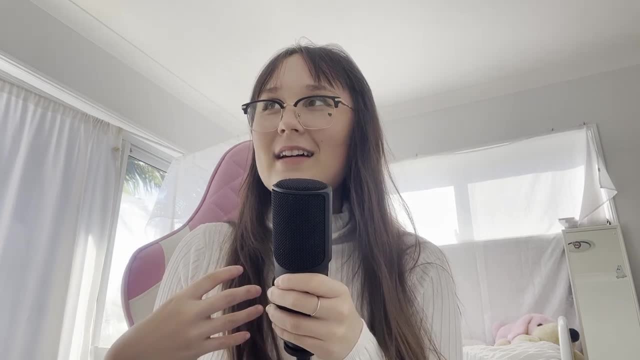 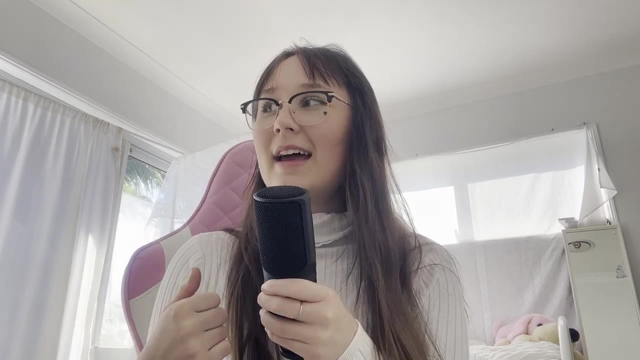 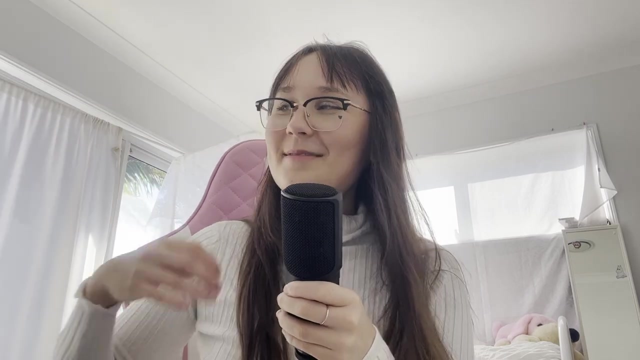 in a cyberpunk sort of vibe, where an assassin, yeah, is like like what I have to protect this petty stuck-up prince, but it he does it for the money you know, and yeah, he ends up like having to protect him from like the assassins in the sort of city, um, and they kind of like band together maybe I. 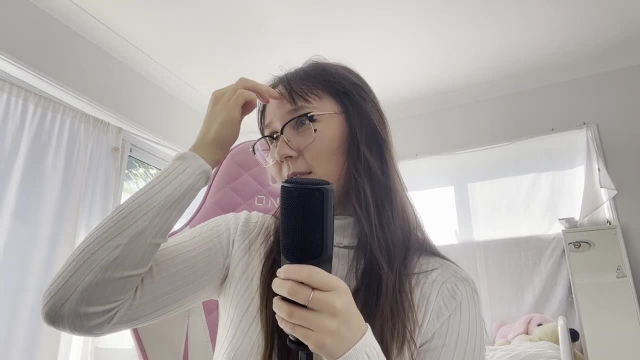 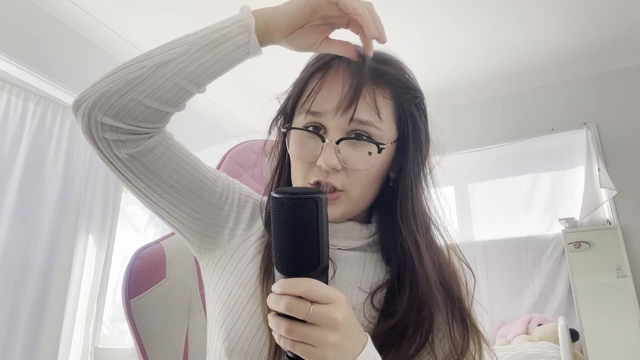 don't know, it just seems kind of intriguing. so that's that one. next up, we have a rebellious witch who steals an ancient relic from her academy. this is actually sorry, I keep playing with my fringe. this is actually a short story slash book that I had. 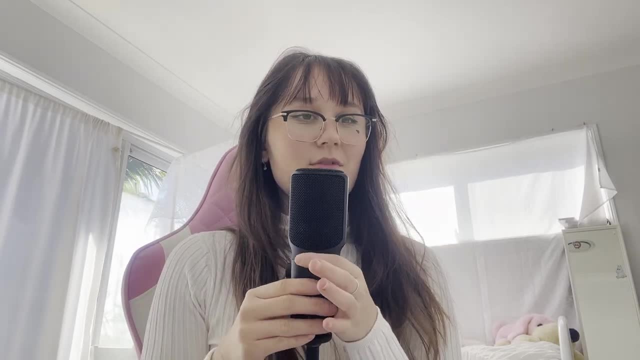 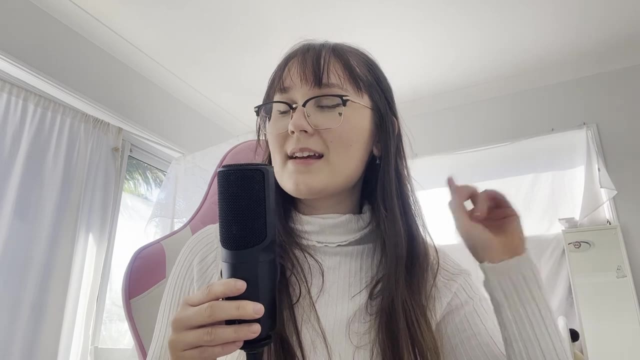 a vlog on. I think I just randomly wrote like the first few chapters of this book and I'm like, yeah, I'm gonna write it. but then I kind of like burnt out. but this was kind of like the premise of the story. well, like a cool witch, yeah, literally. I think she kind of like puts a curse on or like. 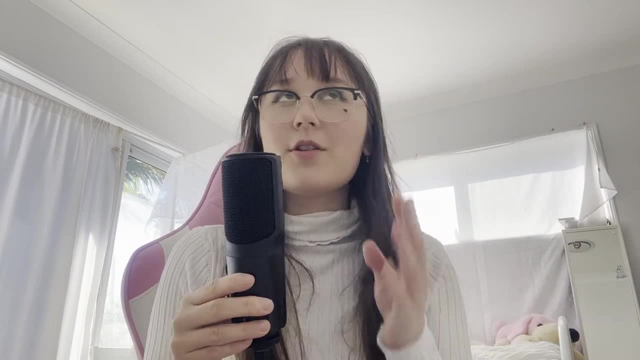 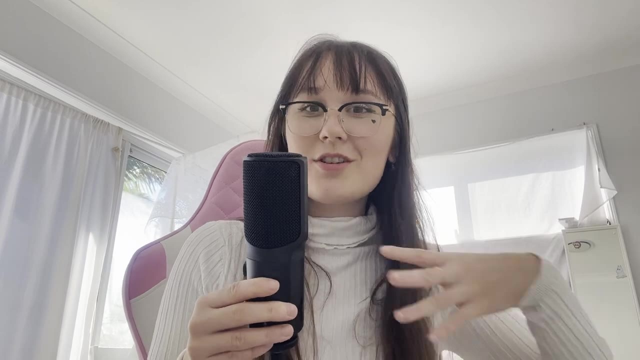 stealing the relic. it was like a book of curses, no, a book of curses, a book of spells that ended up becoming curses, because she ended up writing her own spell, which turned into a curse, which cursed everyone to forget her name, but for some reason, one boy from 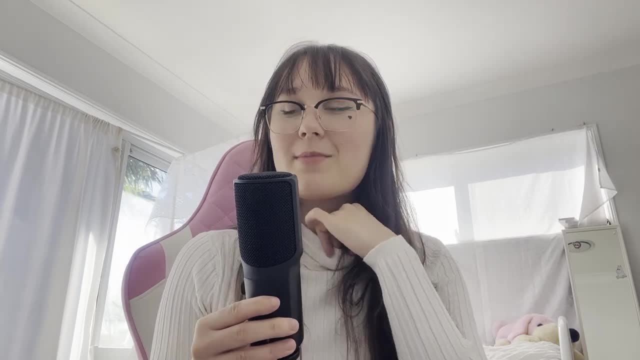 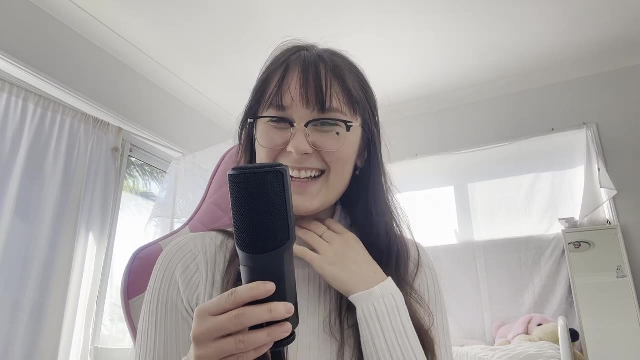 the academy remembers her name. so that's kind of like where the story started. but I'm like I don't know, it wasn't the most pressing sort of book um idea that I had, but that's that okay. next up we have a group of friends who get stuck. oh no, a group of friends who get sucked. 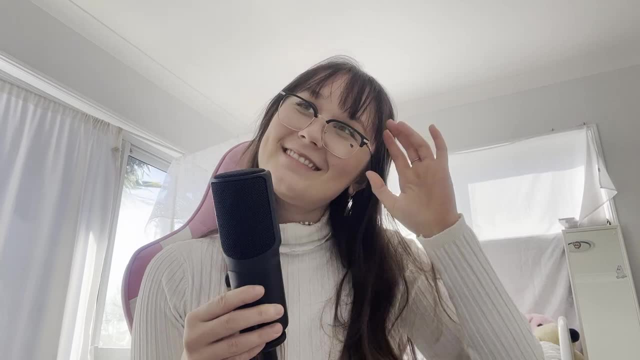 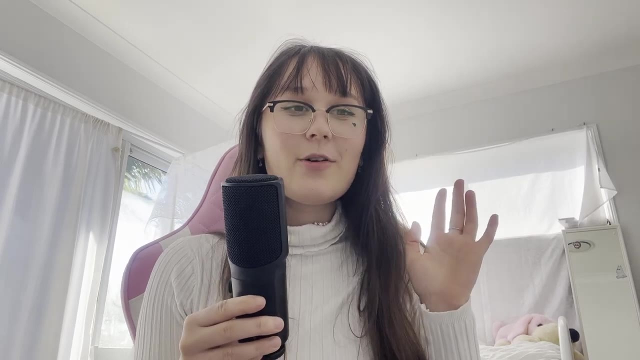 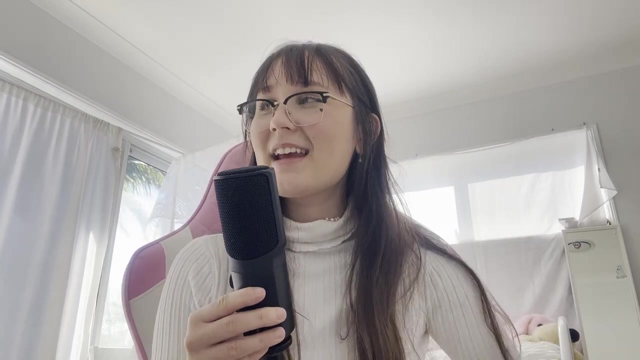 into a book in a forgotten school library. oh, this seems really fun, like, or maybe they get like um, transported into like a series of books or like different books and they kind of meet each other at the end and like they kind of- oh, I don't know, it seems cool, like when they intersect or something, um, but I don't know, I've 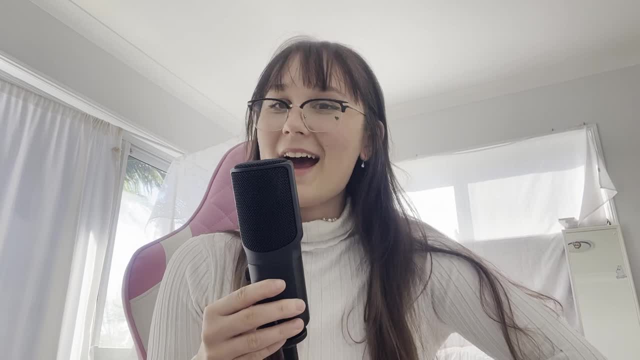 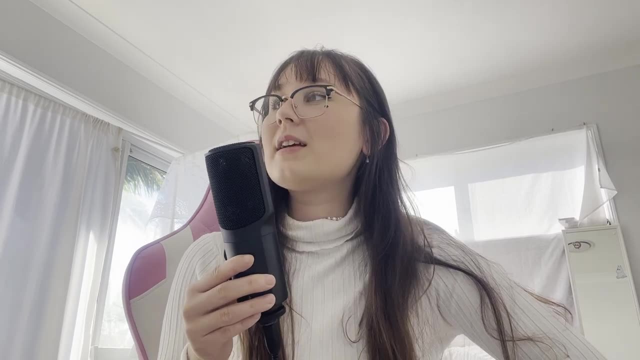 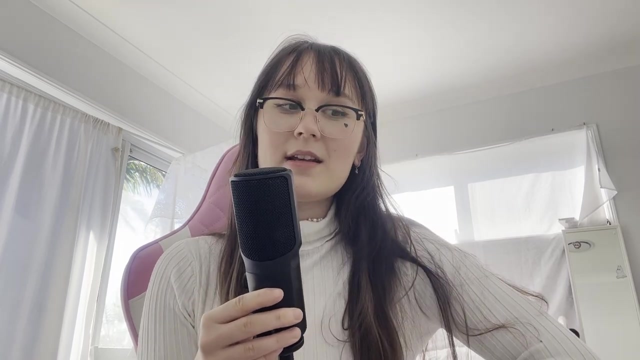 always wanted to write or read a story where this happens, where, like I, can get sucked up into a book and like walk along its characters. I just think that would be so entertaining. okay, next up, we have a hooded maiden who steals the eyes of her captors. so maybe this maiden is like someone who 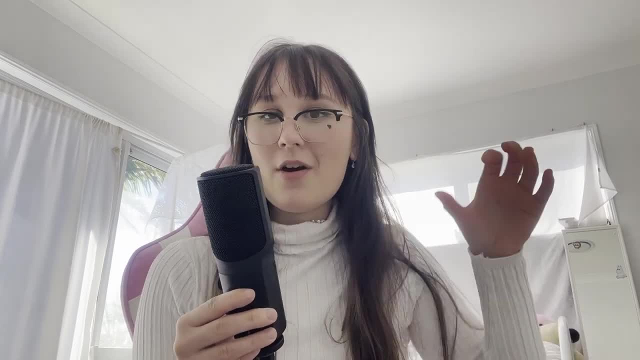 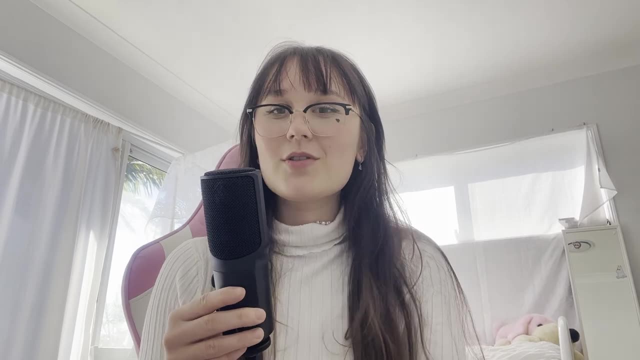 attracts people, attracts men, but she ends up stealing her eyes, stealing their eyes, I don't know. seems like a very interesting sort of um story, very like more of a short story I kind of get the vibe from. but she obviously steals them for a reason, a wholesome reason, I hope. um, that's. 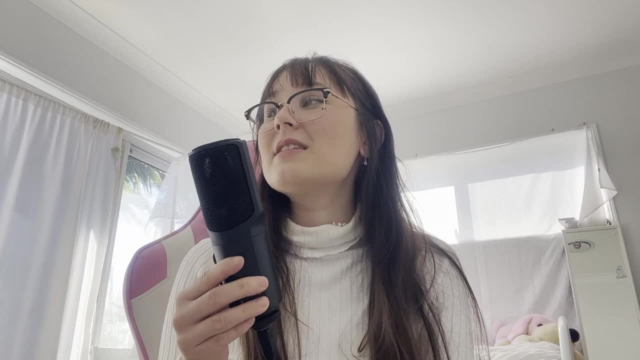 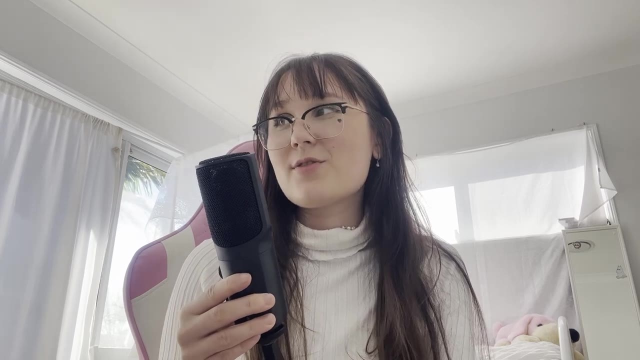 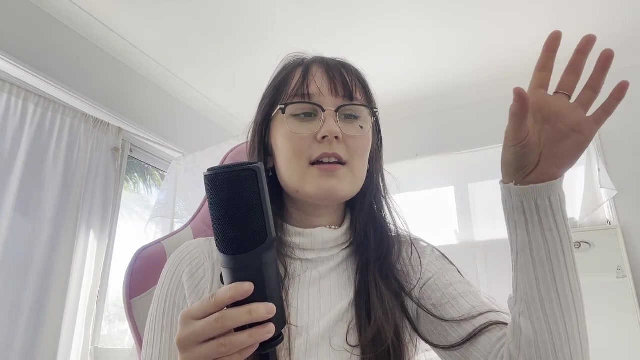 that. and then we have next up a dark, ancient um being saved by a little girl in the forest when she's led astray. I kind of saw this image of like a little girl like outreaching her hand to a like dark beast. that kind of looked like a shadow sort. 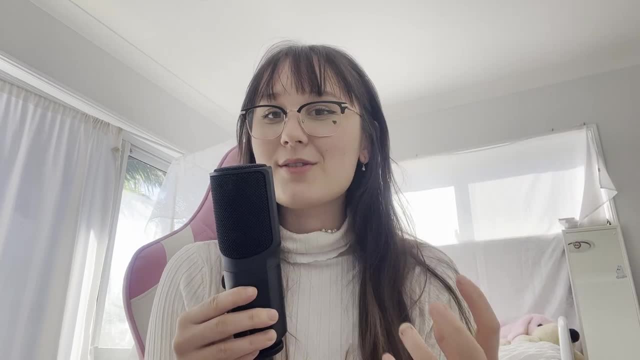 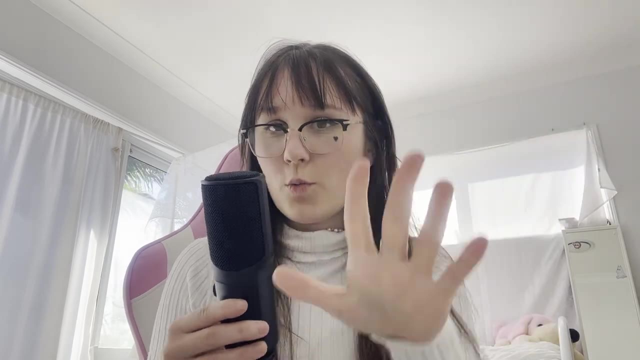 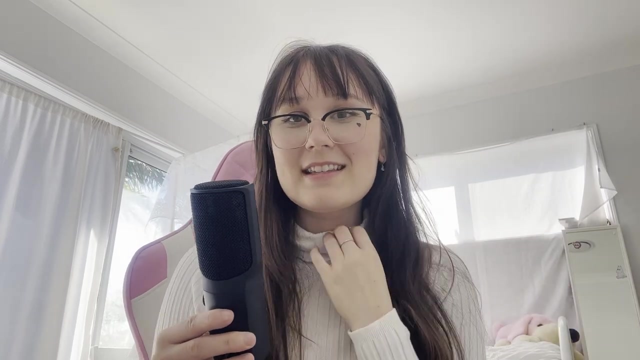 of dragon. so how cool would it be. I love those relationships too, where it's like a huge beast with, like such an innocent child. um, not that, not in a weird way, of course, but more so in like the dark, big, you know creature is wanting to care for this innocent babe. 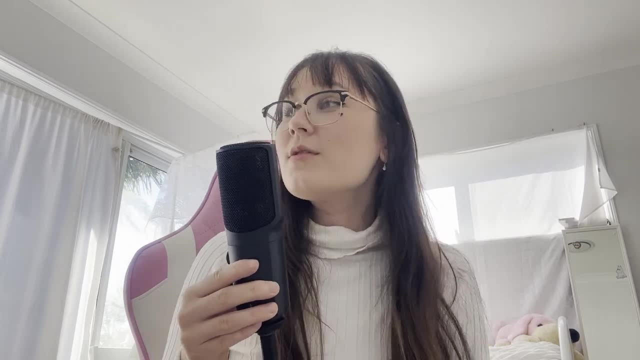 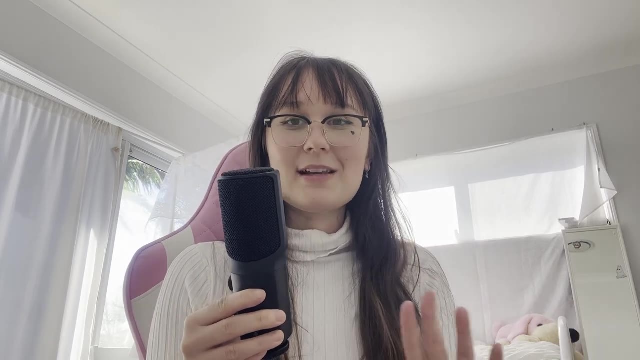 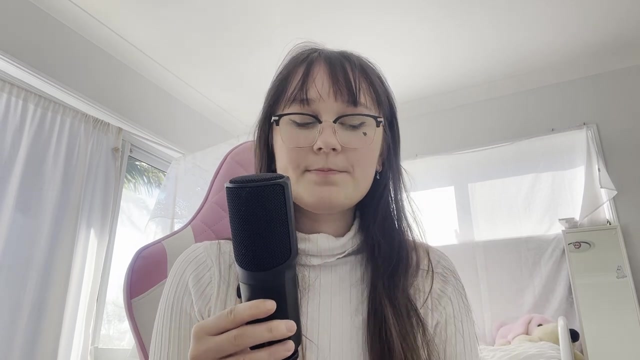 so that's that next up, we have two lovers with the powers of light and shadow and um, they're banished from each other. so these two lovers are basically banished, maybe like heaven and hell, something like that I was thinking of, like shadow and like lightning and storm, you know some sort of 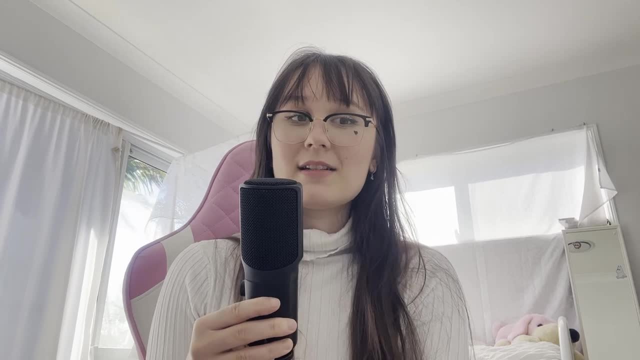 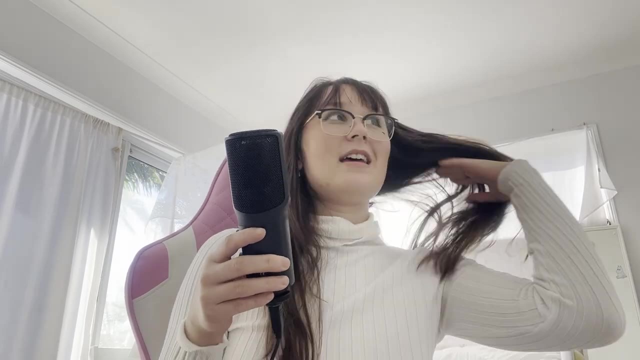 elemental restriction, uh, but light and darkness seems cool in like a dystopian world where it's all darkness or all lightness or something like that. um, and it's just like everything happened because of these two lovers and they were somehow broken apart. so yeah, next up. 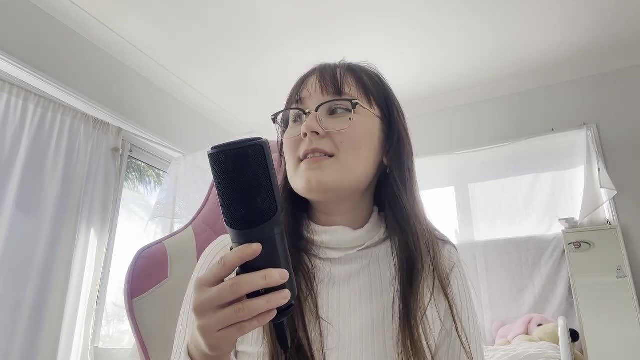 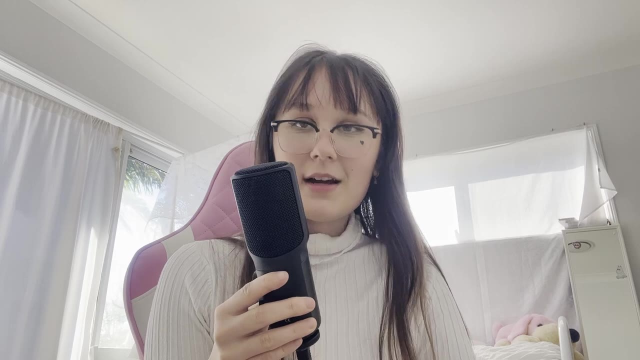 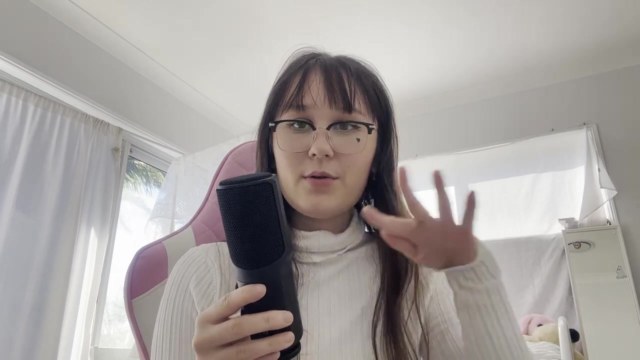 we have two cousins who fall into a puddle that leads to the underworld. I got inspired a little bit from Narnia, the first book, um, in the Narnia chronicles. I love that book so much, it's so good. um, and I just, you know, there's like the world between worlds and there's like all these puddles. 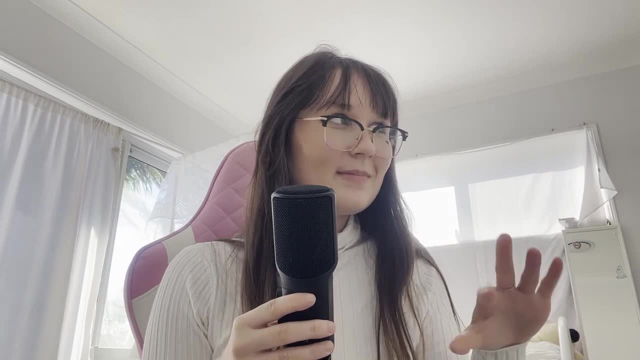 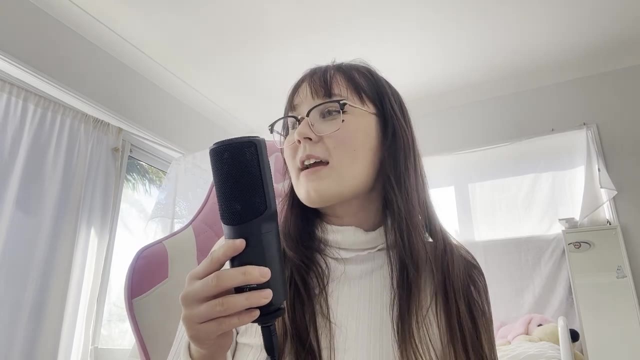 with guinea pigs. there's guinea pigs running along in the little little grass, but that's kind of like what I inspired, what inspired me, but that's a kind of cool, fun idea. okay, the prince, this is a good one. I hope you've like stayed till this one, because this one I was kind of proud of um. 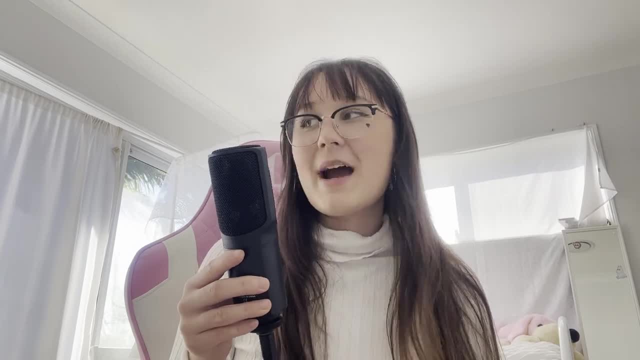 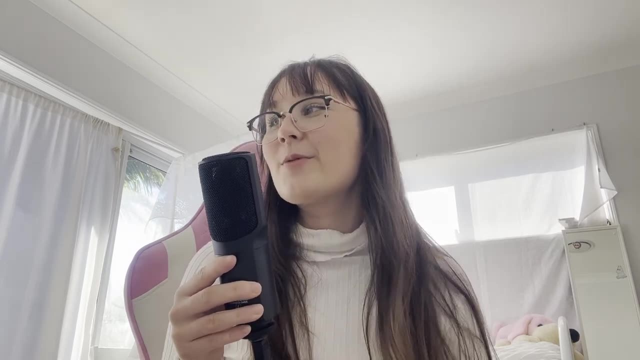 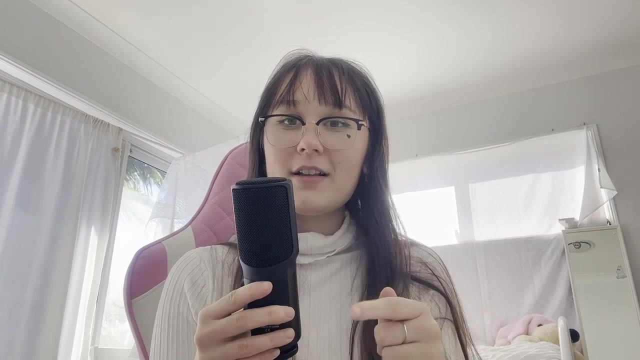 so the prince is running away from his marriage only only to meet the woman he was supposed to marry, a woman who happened to also be his assassin. how cool like the prince runs away because he was about to marry a girl he didn't want to, but it turns out like that girl was. 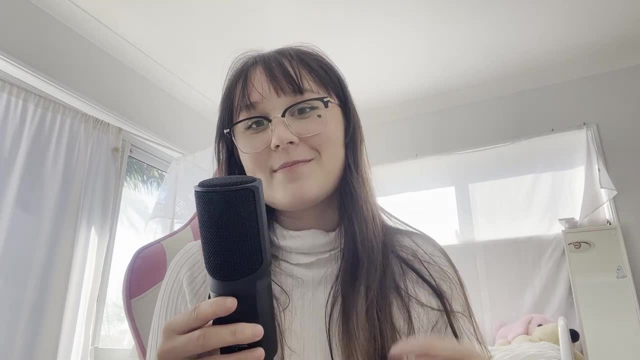 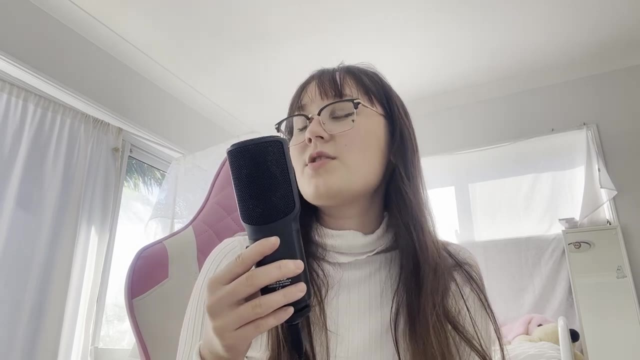 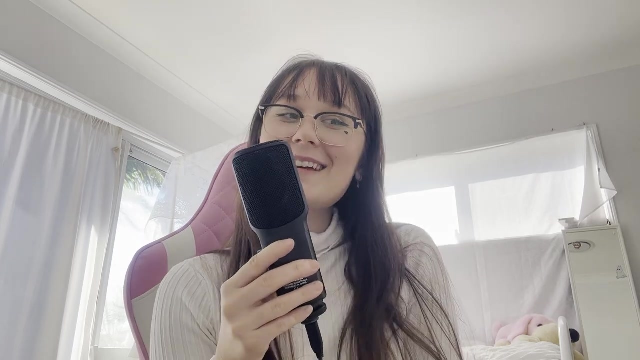 trying to kill him and then he ends up running away, which is a good thing, but then maybe they like learn about each other. I don't know, something like that. okay, next we have bored drunk students stumble into a graveyard and find their names on a tombstone. this one was Loki, like right up my 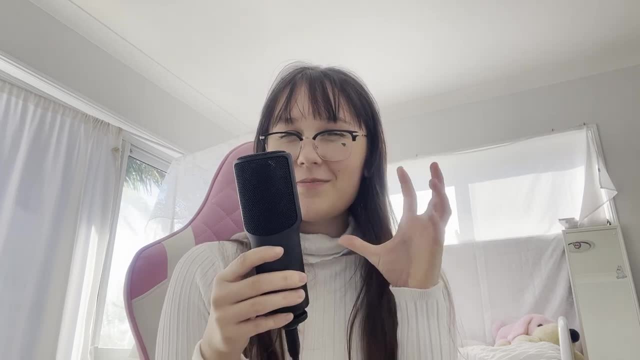 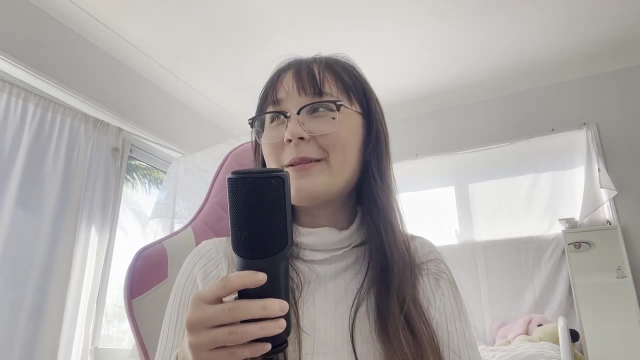 alley, I love books that kind of seem like this and just like very like mystical, ghosty sort of um shadowy things are just untangible and it's all like gloomy and like just like weird. I love those sorts of books. oh my gosh, okay, next up a struggling. 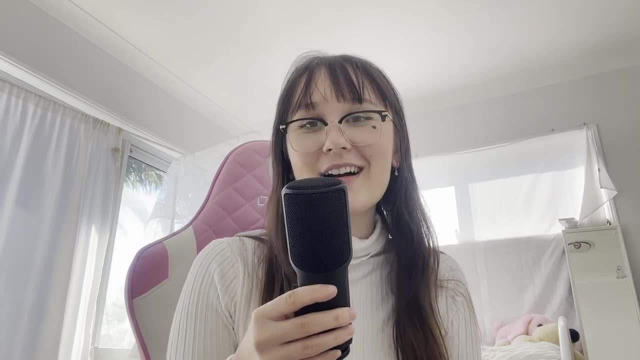 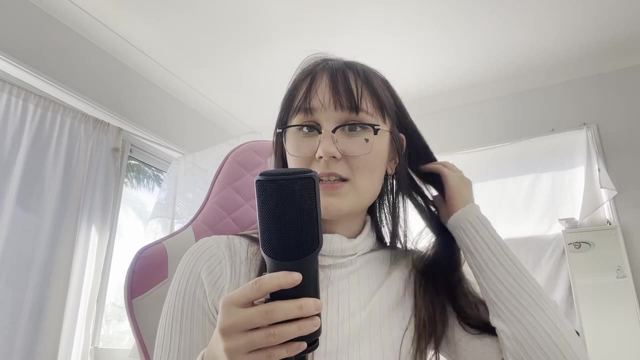 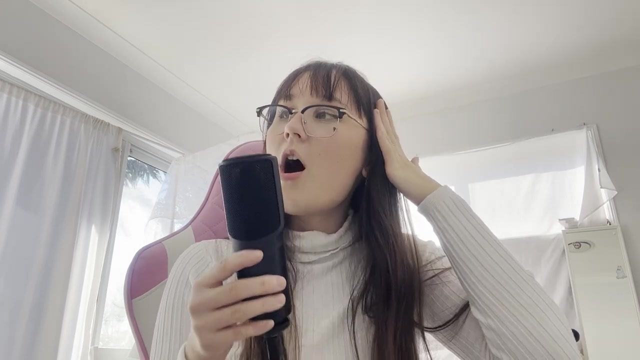 writer is cursed by a ghost who claims he is her lover. this is interesting, kind of inspired by Cassandra Clare's last hour series, where there's the character Jessie and Lucy, who's the character? she is a writer and then she falls in love with a ghost. but perhaps this, oh, maybe, like the writer. 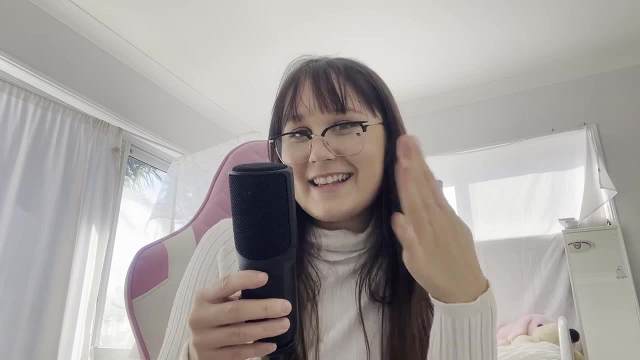 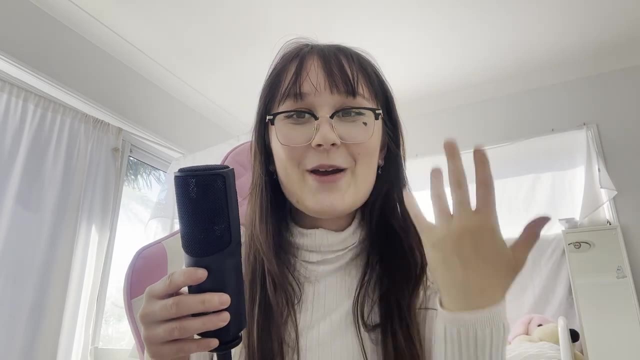 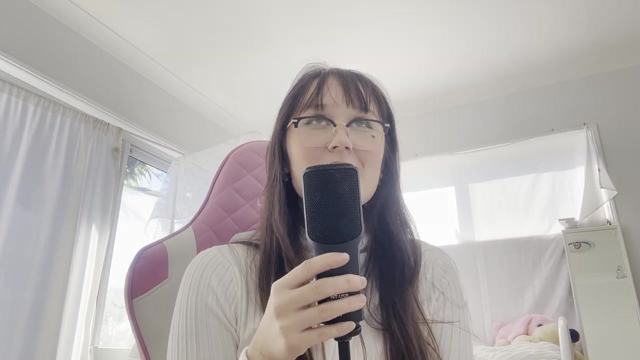 is writing a story about two lovers and then that's them. I don't know something like that. it's kind of weird, messed up, but hey, it's a book idea. there you go, okay. next up we have a pirate son who saves a merman boy from the nets, because usually it's the mermaid serving saving the the. 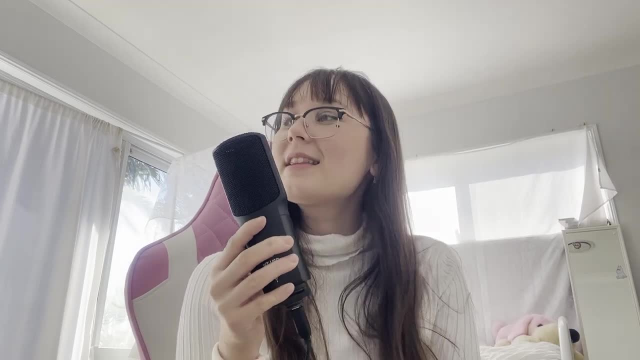 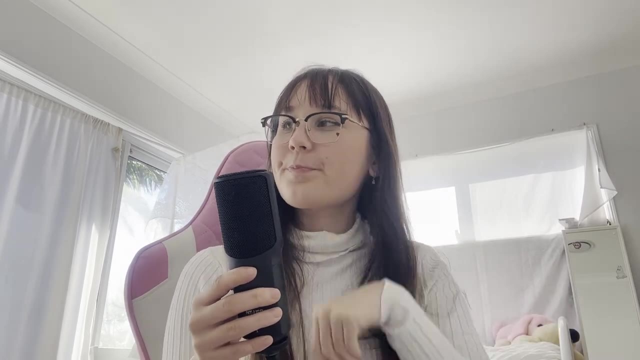 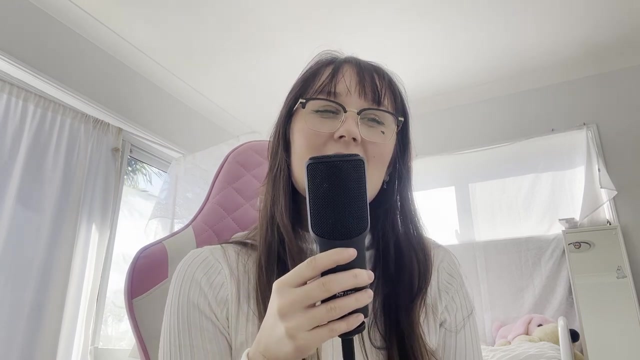 pirate, right, or the, or Prince Eric, whatever. I would like to see a pirate saving like a mermaid or a merman. I think that'd be so cool. um, and yeah, that's that one. next up, we have an artist who falls in love with the girl in his painting. this seems like more of a short novella sort of thing, where 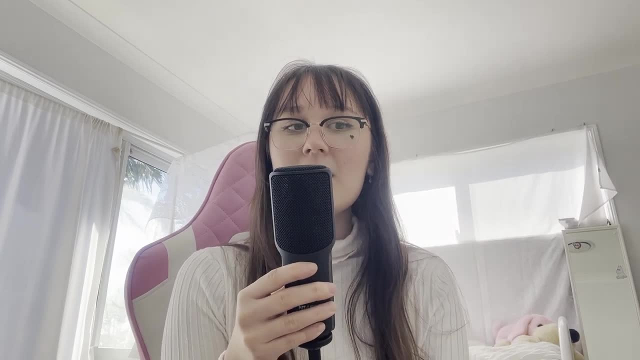 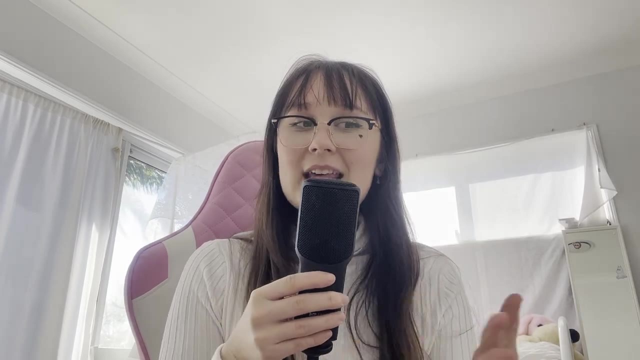 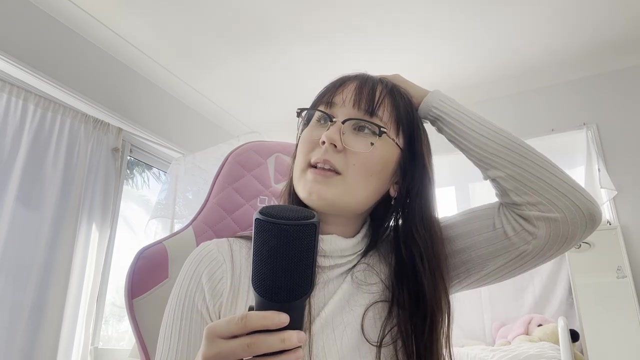 someone gets so obsessed like the painter, gets so obsessed with their artwork and like so attached to the character they've um painted that you know sorts of things. blur like reality and um fiction, blur like. I think that would be such an interesting read. I love objective like weird stories like this. 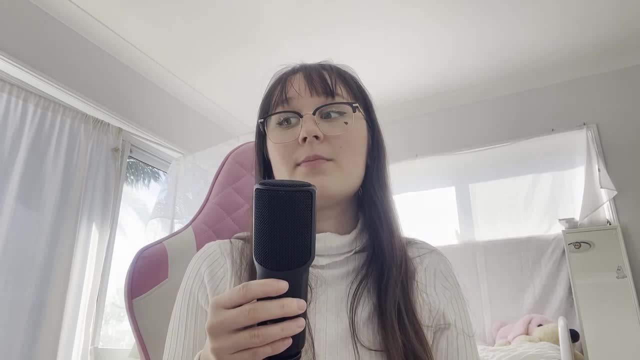 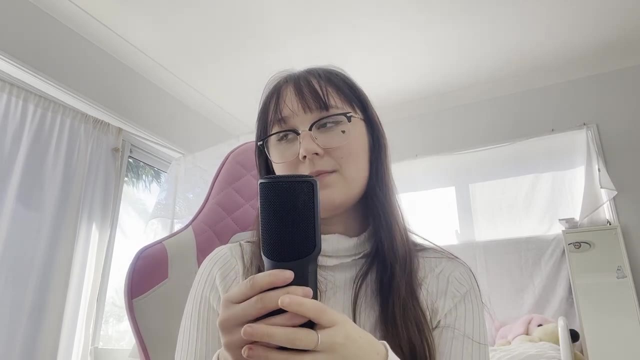 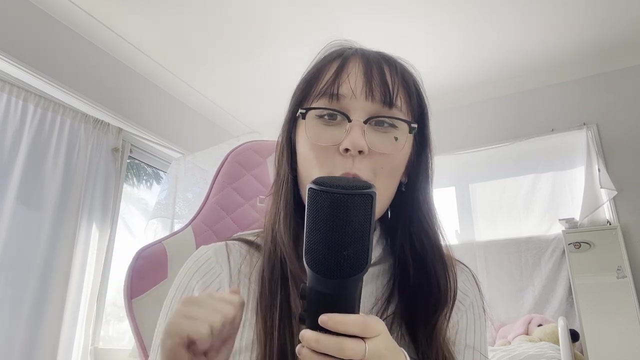 like this. this sort of idea reminds me of um Piranesi by Susanna Clarke, which is a book that's my favorite book, so I love ideas like this. okay, next up, we have a two-faced scholar who takes his class on a sinister excursion to another world. how cool would that be like? it kind of reminds me of. 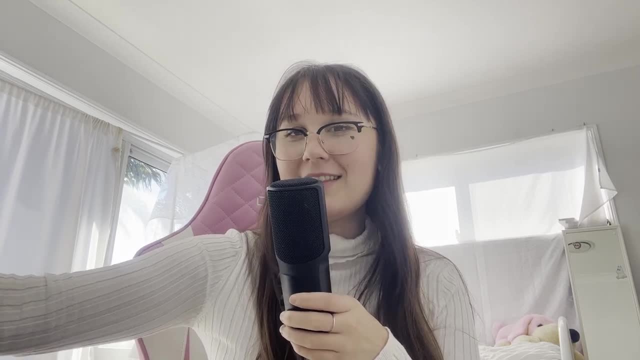 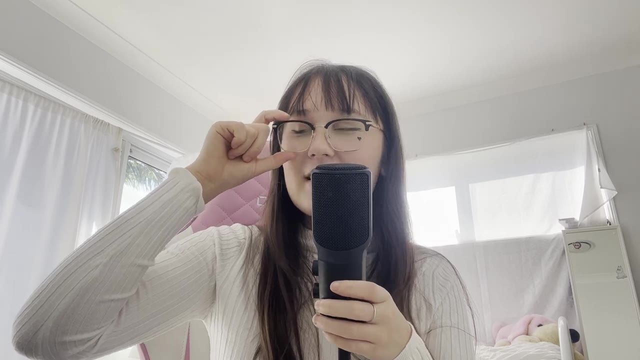 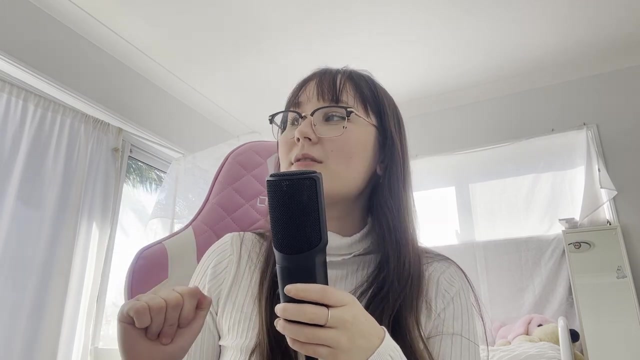 Snape, someone who would like just do something weird and like. it's not who you seem like. where do they go then again, it kind of reminds me of the magic school bus. is that what it's called? I forgot the theme song, but anyways, last one. we have a deaf pianist who can see notes instead of hear them, or like they can sort of see notes. 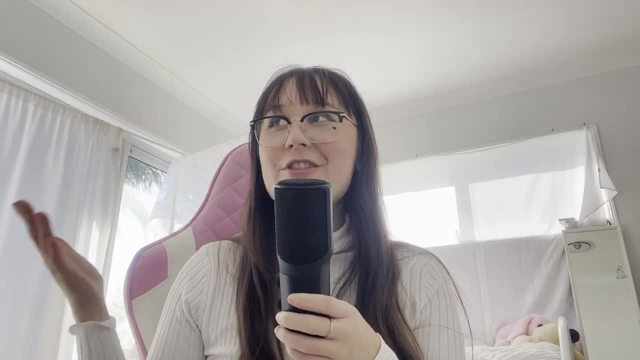 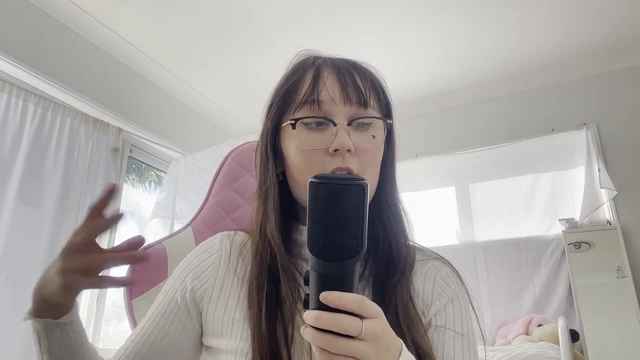 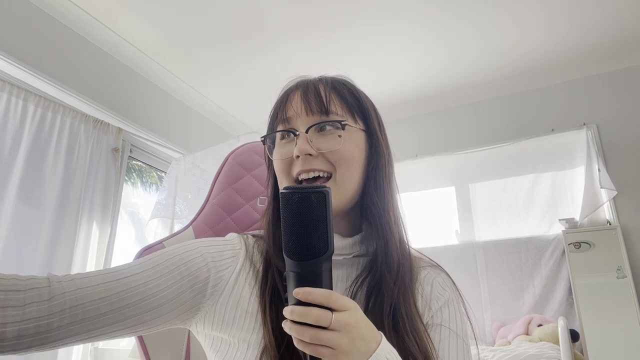 in their mind as colors or as visions, and I did get inspired from Project O, which I'm actually writing at the moment, did some writing on that last night and I'm really excited. I'm actually so in a good place with this book. so, um, that was kind of inspired by Project O, but that's. 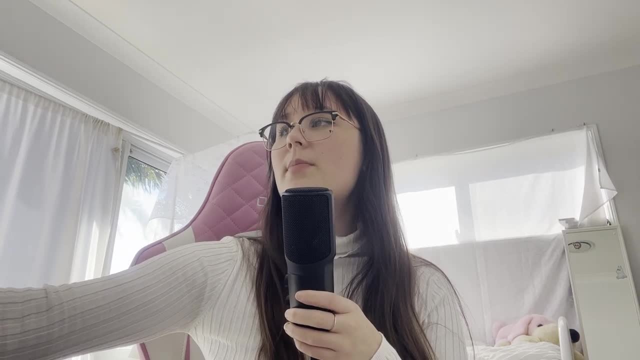 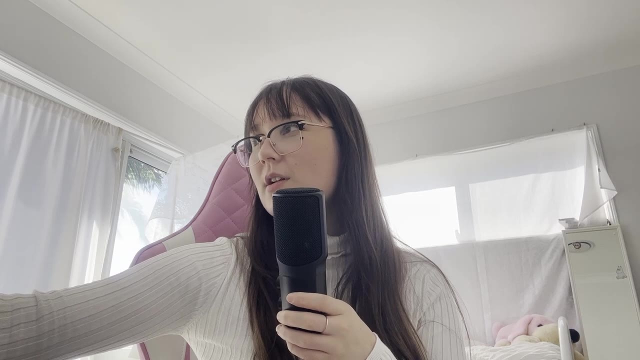 all of them. I literally don't know how many there are, but I had a lot of fun just talking about everything and just seeing if, um, I actually want to know how many there are so I can put in the title of the video. give me one second. 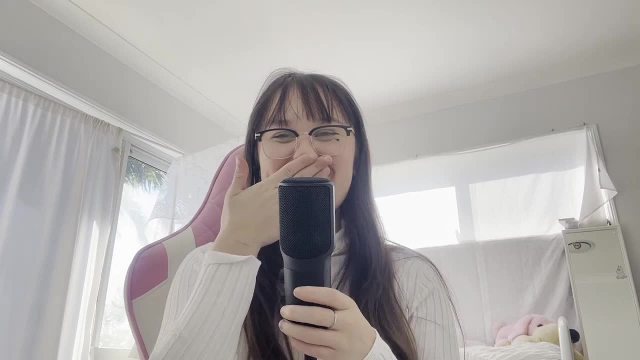 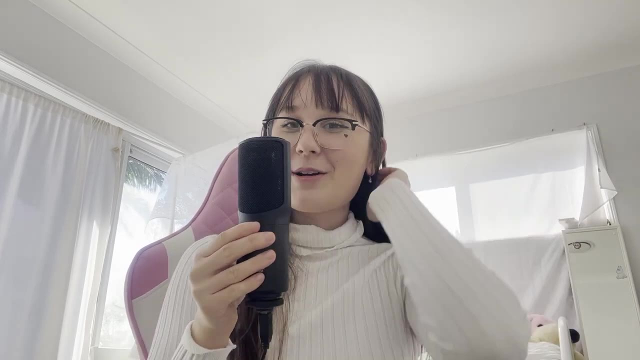 there will, oh my gosh, literally 20. I was right, wow. ah, that feels like surreal moment. I'm so smart, sorry, um, I had so much fun just talking about my ideas and I hope you got inspired or just enjoyed kind of just talking about it and just letting me. 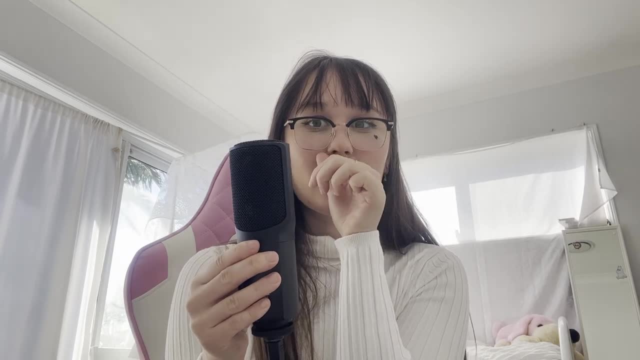 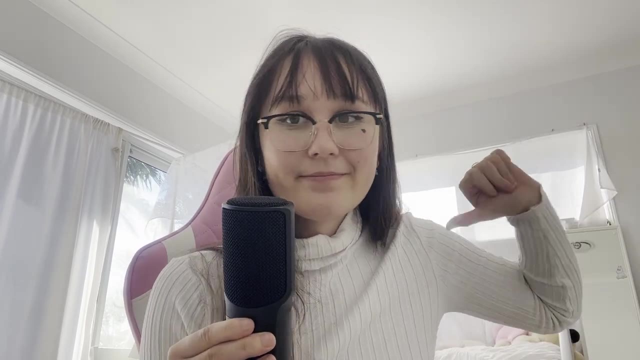 speak about it. I hope that was helpful and I hope you guys enjoyed it and I'll see you guys in the next video. bye, about some ideas i have and i literally just came up with all of these, or most of them, just like on the spot. so if you want some more book ideas, come to me, but take them, as you will include some of. 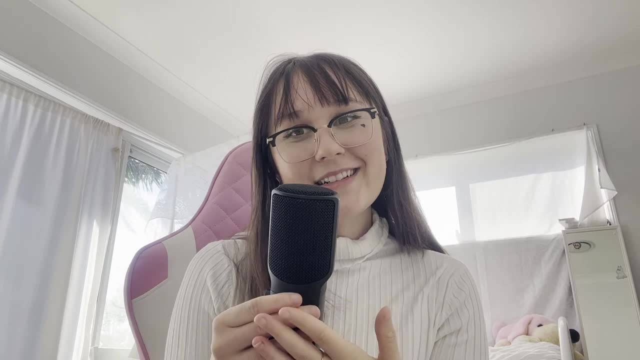 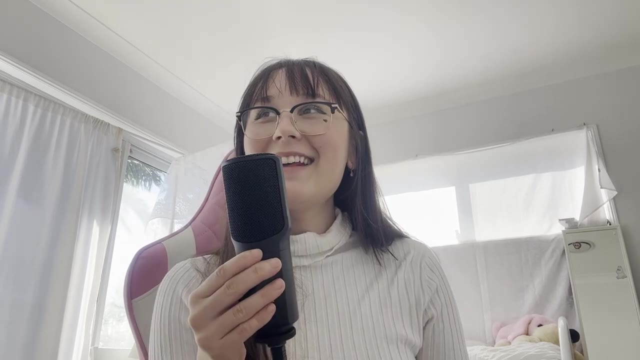 these tropes, some of these characters in your books, and let me know how you feel, or maybe just write a short story about these premises. premise, i promises, promises, i think. um, anyways, again, definitely check on my instagram. i post there so frequently if you want updates on my, about my book. 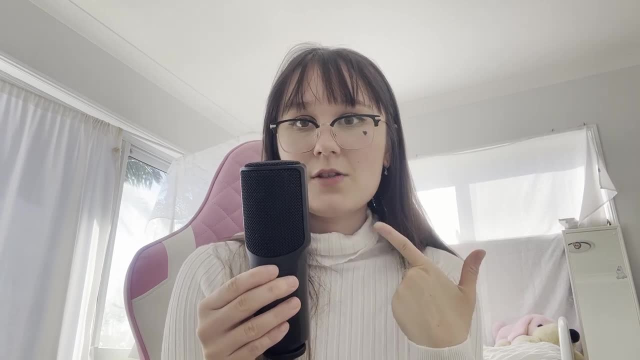 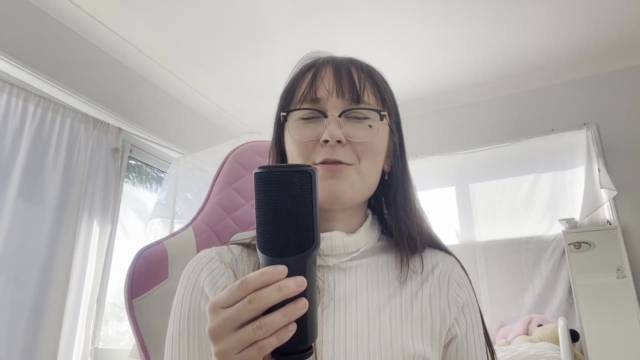 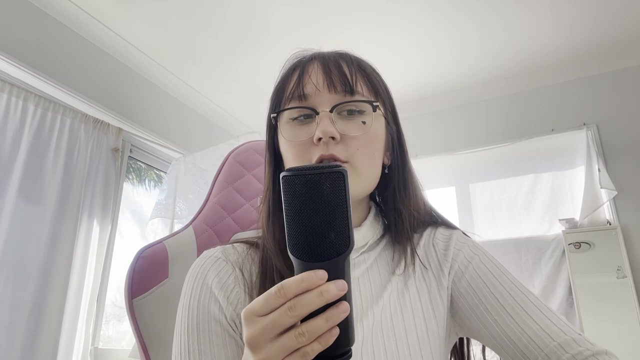 about, like what i'm reading about, but everything it's on my instagram and also discord- y'all. we are upping the discord game. um, i write every there. i write every there. i write there every single week on wednesday at wednesday 6 pm est. i'm not sure if i'm gonna be changing that because uni's coming. 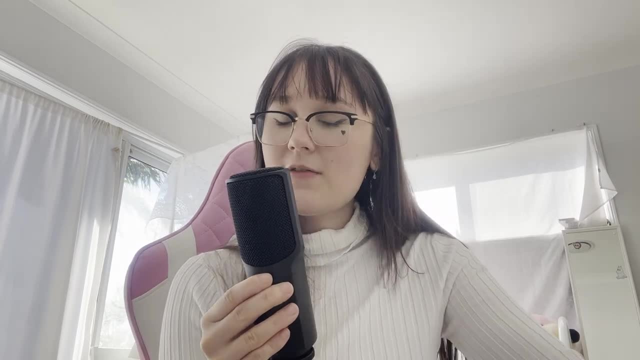 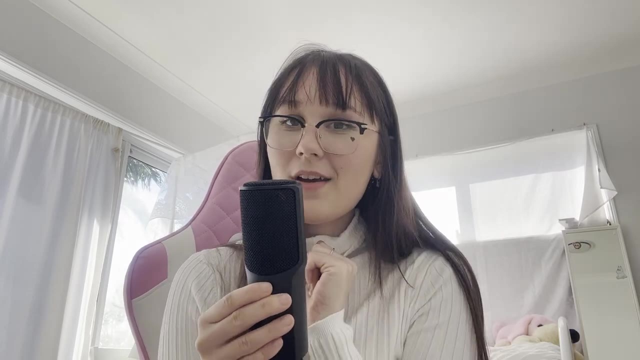 up um, but i'll keep you guys updated. but just know, if you want to find a writing buddy, someone to write with, if you've always wanted a writing friend, go to discord, because it's a i built for you guys so you guys can come together and get inspired from each other. but 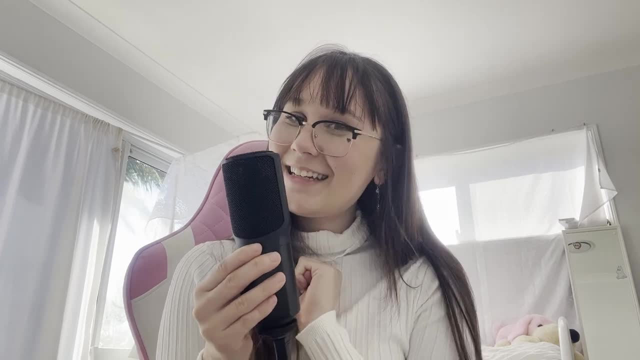 anyways, i hope you're inspired from this video and i hope to see my next writing podcast. bye everyone.